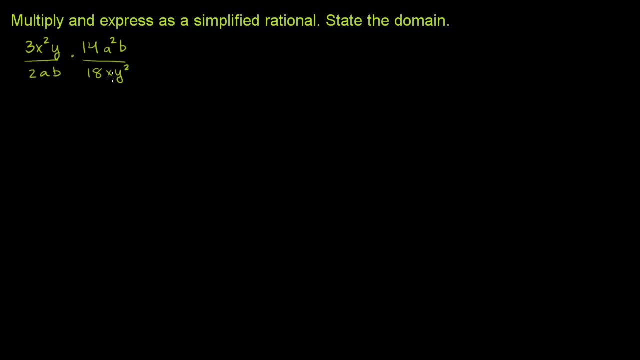 when either a, b, x or y is equal to 0. If any of those are equal to 0, then we have an undefined expression. So we could say that the domain is all real- a's, b's, x's and y's- except 0.. 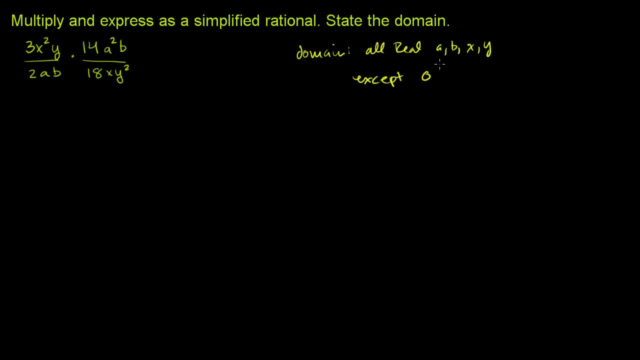 Or we could be specific, except a, b, x and y can't equal to 0.. Or you could write maybe this: Given that a, b, x and y can't equal to 0.. x and y does not equal 0. 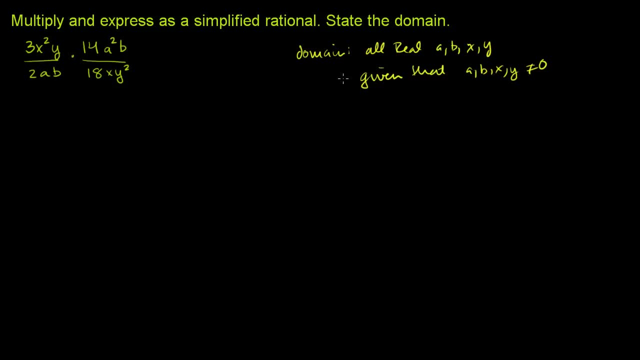 That none of them can be equal to 0. These are just multiple ways of stating the same thing. Now, with that stated, let's actually multiply and simplify this rational expression. So when we multiply, you just multiply the numerators and multiply the denominators. 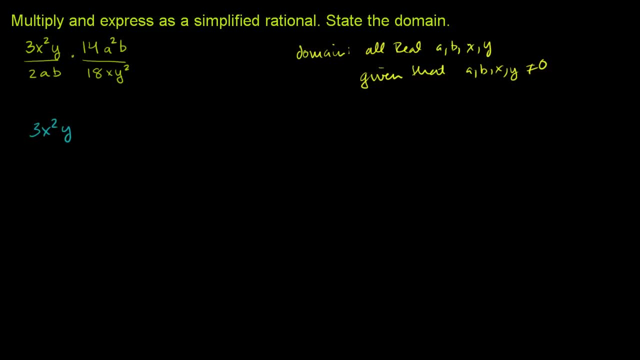 So you have 3x squared y times 14a squared b in the numerator and then in the denominator. we have 2x squared y times a squared b in the numerator And then in the denominator. we have 2x squared y times. 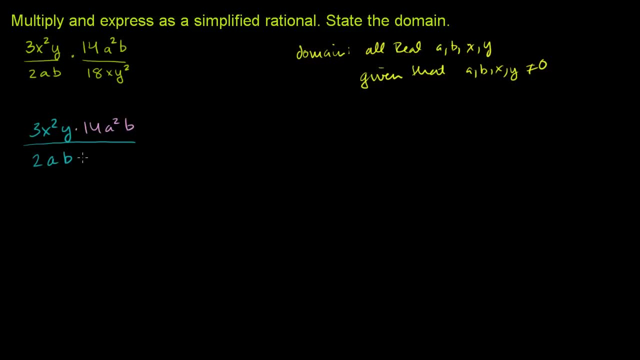 2ab times 18xy squared. And let's see where we can simplify this thing. Well, we can divide the 14 by 2 and the 2 by 2.. And see what we get: 14 divided by 2 is 7.. 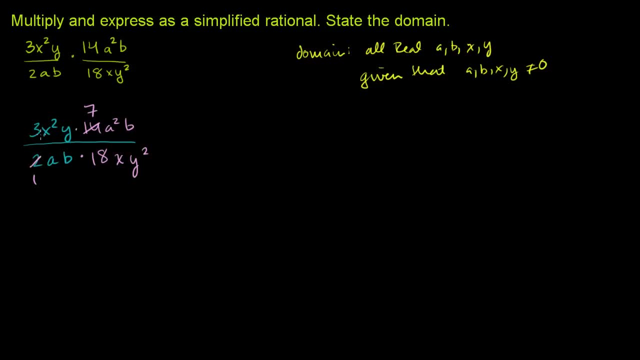 2 divided by 2 is 1.. And we could divide the 3 by 3 and get 1, and divide the 18 by 3 and get 6.. Every time we divided the numerator and denominator by 2, now the numerator and the denominator by 3.. 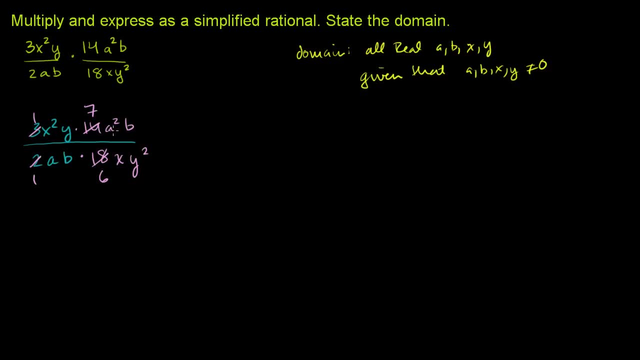 So we're not changing the expression. And then we can divide a squared divided by a. So you're just left with an a in the numerator And a divided by a is just 1.. You have a b over a b. Those guys cancel each other out. 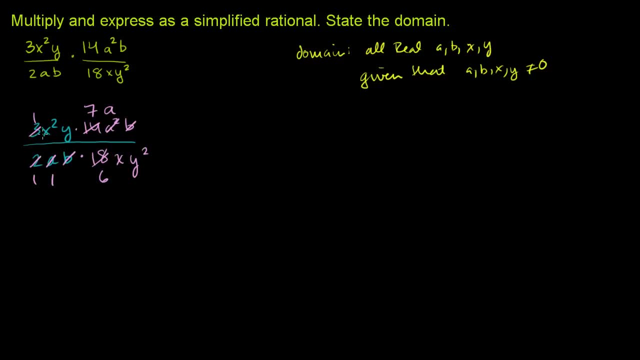 You have an x squared divided by an x. So x squared divided by x is x, And x divided by x is just a 1.. So it just becomes an x over 1, or just an x, And finally you have a y over 1.. 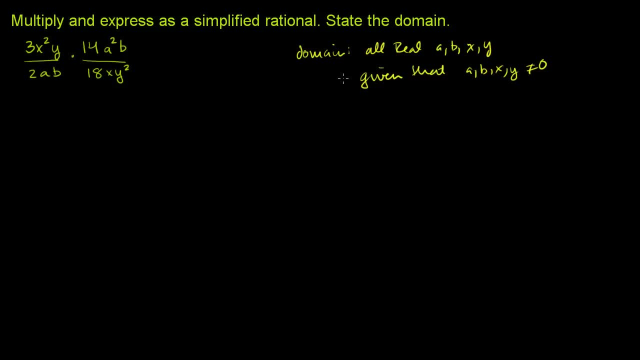 That none of them can be equal to 0. These are just multiple ways of stating the same thing. Now, with that stated, let's actually multiply and simplify this rational expression. So you just multiply the numerators, multiply the denominators. 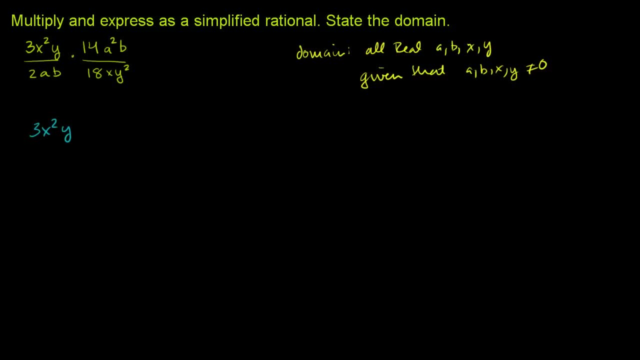 So you have 3x squared, y times 14a squared, b in the numerator and then in the denominator we have 2ab times 18xy squared. And let's see where we can simplify this thing. Well, we can divide the 14 by 2 and the 2 by 2.. 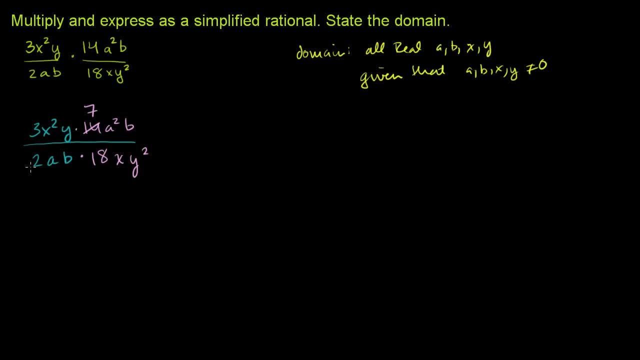 And see what we get: 14 divided by 2 is 7.. 2 divided by 2 is 1.. And we could divide the 3 by 3 and get 1, and divide the 18 by 3 and get 6.. 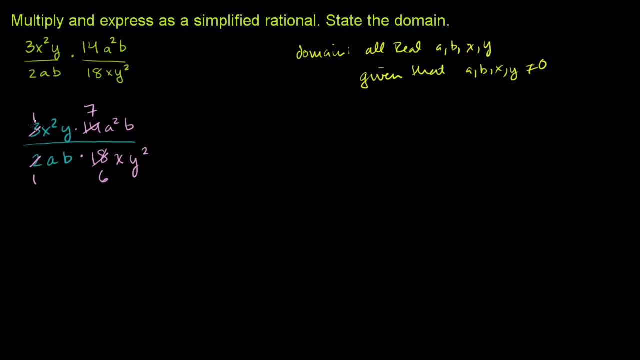 Every time we divided the numerator and denominator by 2, now the numerator and the denominator by 3.. So we're not changing the expression, And then we can divide a squared divided by a. So you're just left with an a in the numerator. 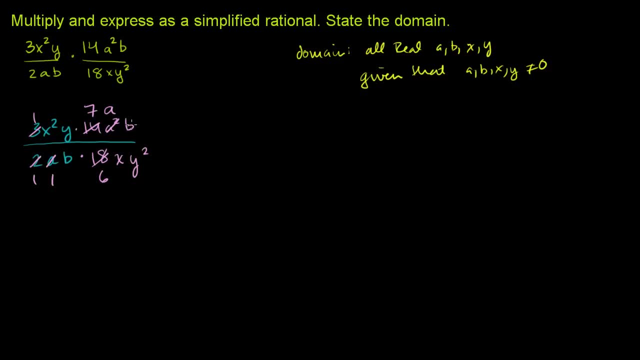 And a divided by a is just 1.. You have a b over a b. Those guys cancel each other out. You have an x squared divided by an x, So x squared divided by x is x, And x divided by x is just a 1.. 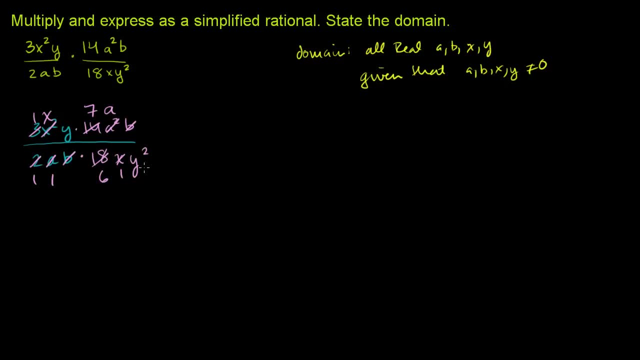 So it just becomes an x over 1, or just an x, And finally you have a y over 1. Or y squared. So if you divide the numerator by y, you get 1.. You divide the denominator by y, you just get a y. 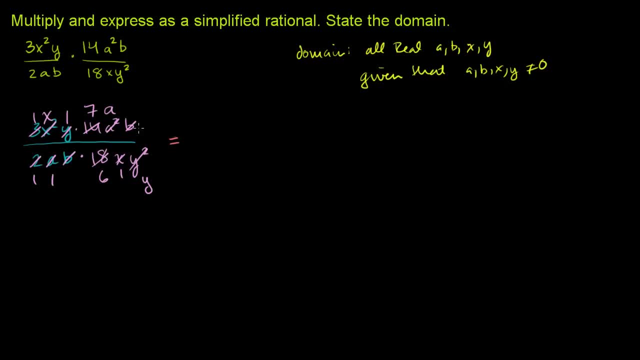 So what are we left with? We are left with in the numerator, all we have these 1's we can ignore. That doesn't really change the number. We have a 7. 7 times a times x. That's what we have in the numerator. 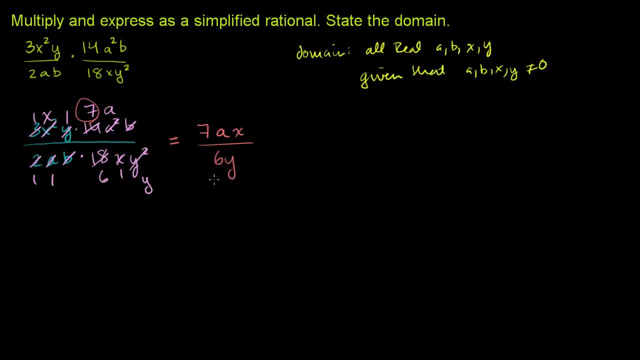 And in the denominator we just have a, 6y And we have to add the constraint That That a, b, x and y cannot equal 0. Because when you just look at this expression right here, you're like, hey, what's wrong with x?